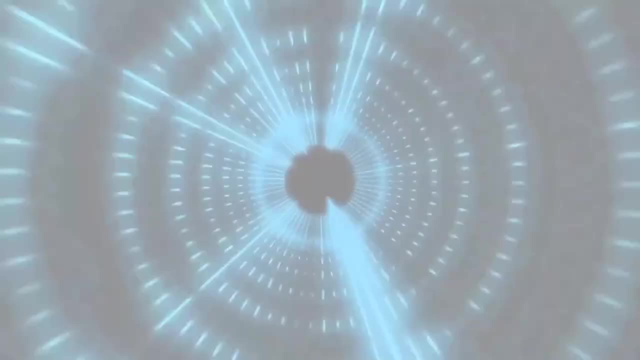 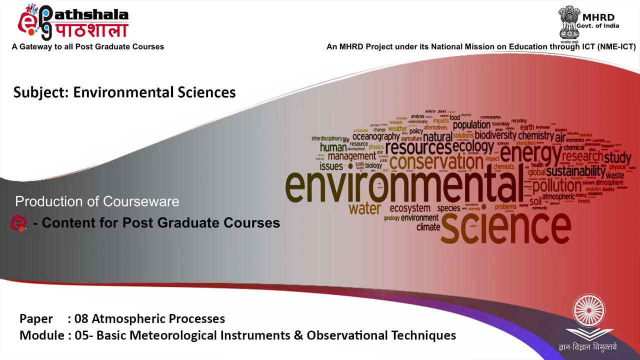 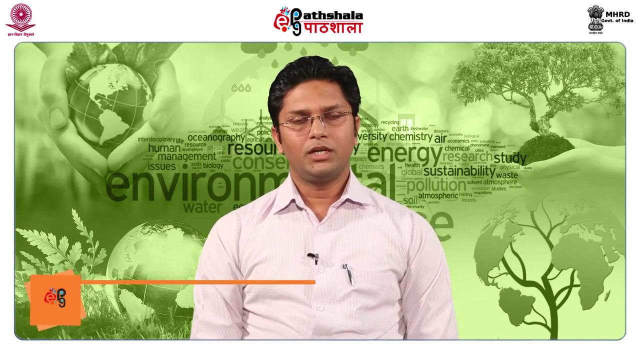 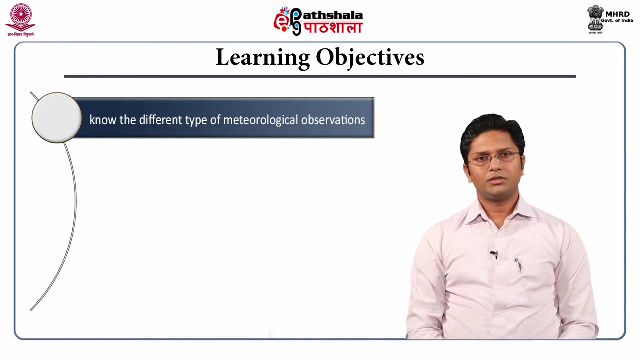 Hello students, welcome to E P G Parsala. In this session we shall discuss on the topic basic meteorological instruments and observational techniques. The learning objectives of this module is to know the different types of meteorological observations, to know about the various meteorological 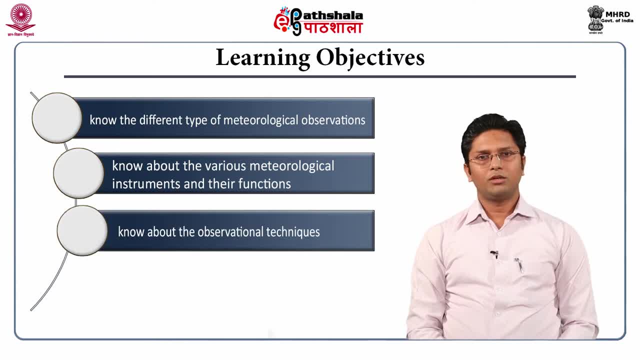 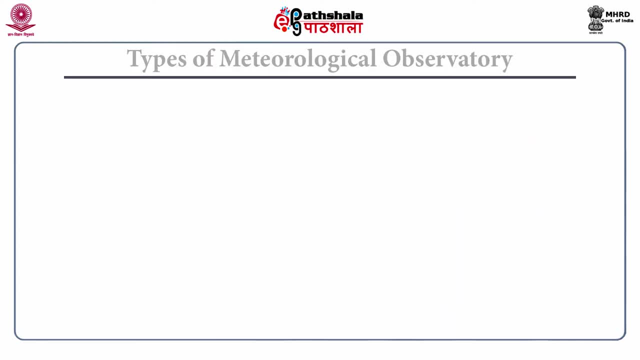 instruments and their functions, to know about the observational techniques and to learn about the importance of each meteorological observation. Let us start with the types of meteorological observatory. One is called surface meteorological observatory. It has six classes: Class 1, where both eye reading and self recording instruments. 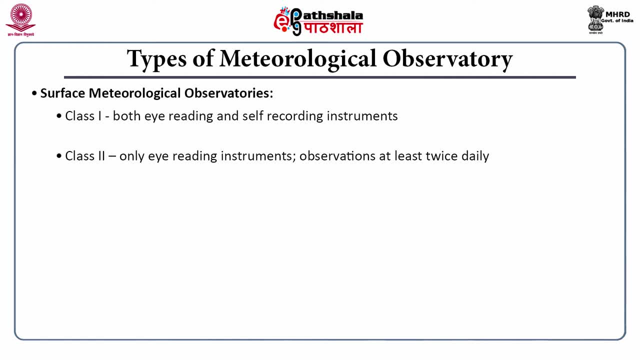 are there. In class 2, only eye reading instruments are there and observations are taken at least twice daily. In class 3,, only eye reading instruments are there and observations are taken once daily. In case of class 4,, 5 and 6, lesser number of instruments are there. 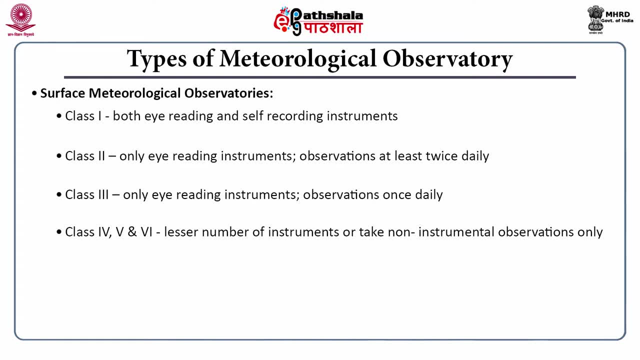 or, in some cases, non-instruments. observations are taken only In case of agronomic observatories. they have been classified into three types: One is principal type, then ordinary and the third one is auxiliary type. Now, what should be the ideal site for the observatory? The IMD, which is the nodal agency? 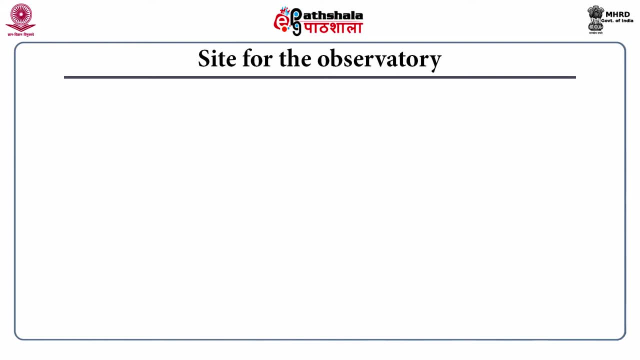 of weather observations and weather services in this country. they have prescribed the standard size, which is 55 meter along north- south direction and 36 meter along the east west direction. A well exposed- it should be a well exposed- bare plot, level plot and 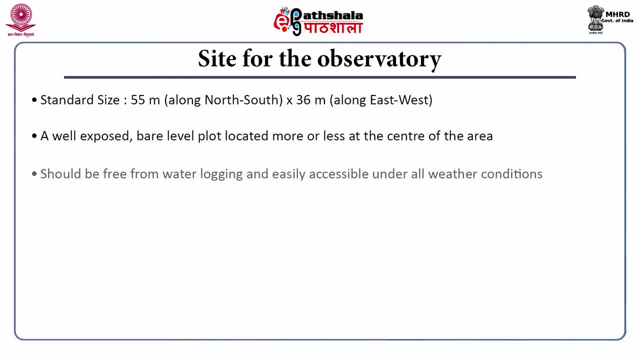 located more or less at the center of the area. It should be from water logging and should be easily accessible under all weather conditions. The soil type of the observatory should be representative of that locality. It should be a good distance away from the large obstructions like tall trees, buildings, main irrigation. 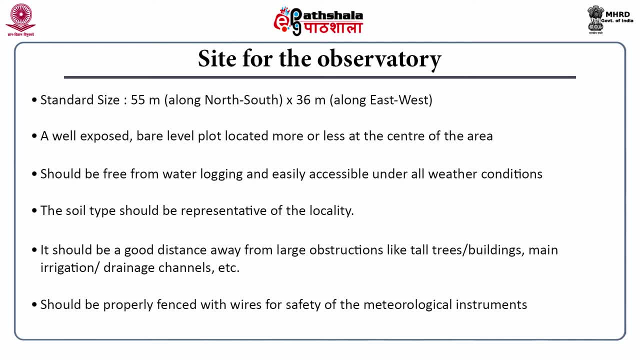 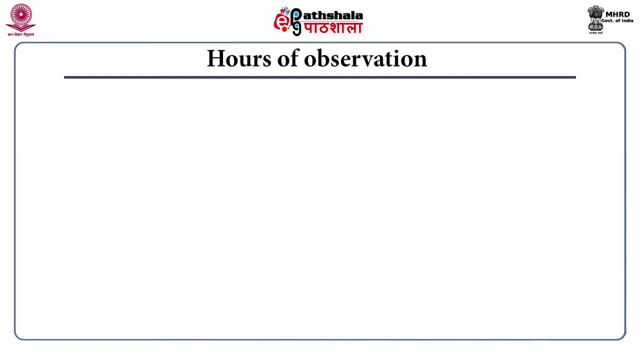 or drainage channels, etc. Also, it should be properly fenced with barbed wires for safety of the instruments as well as free air flow. Now, another important thing is hours of observations. In case of surface observatory, regular surface observations are taken at least twice daily. 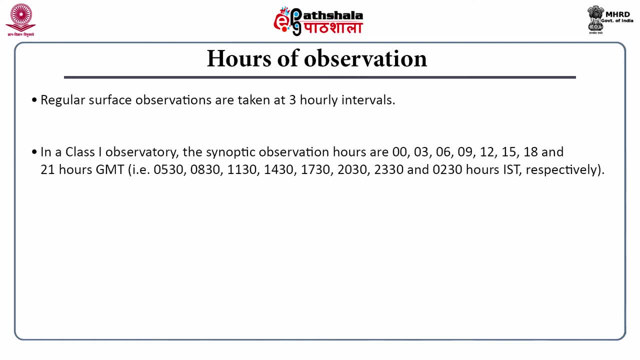 At three hourly intervals. The synoptic hours starts at 0 GMT and then observations are taken at every three hour interval, that is, 6,, 9,, 12,, likewise up to 21 GMT. However, in most observatories in India two observations: one morning observation at 8.30 hours IST and 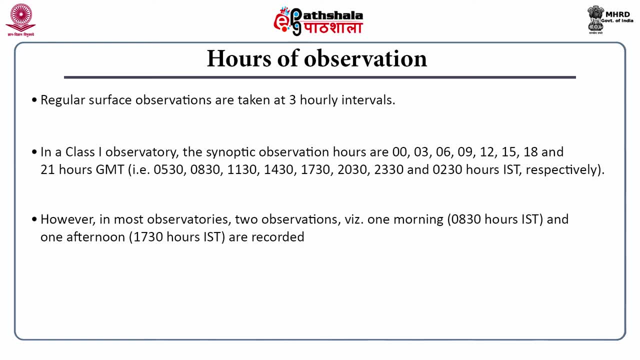 another afternoon observations at 17.30 IST are recorded For agro metallurgical observatories. morning observation is taken at 7.11 am to 7.30 pm. The observation time is approximately, and afternoon observation is taken at 14 LMT. LMT means local mean time. Then in which order? 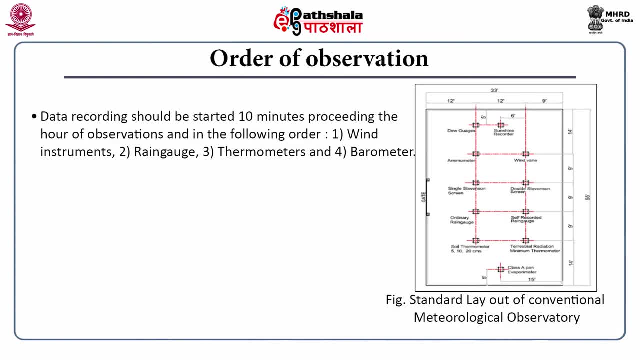 the observation should be taken. Data recording should be started 10 minutes preceding the hour of observations and in the following order: First comes wind instruments, then rain gauge, then thermometers and then barometers. Non-instrumental observations like clouds, visibility, etcetera, should be taken in the interval of 3 minutes of first and second. 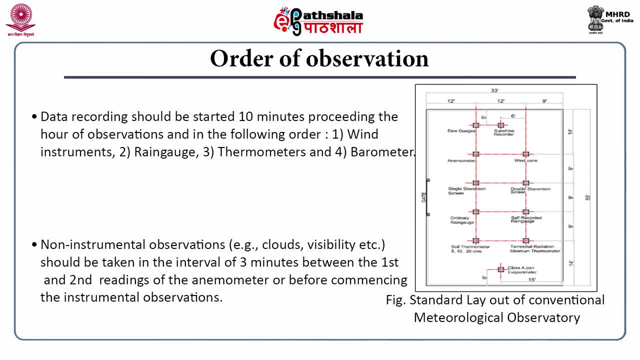 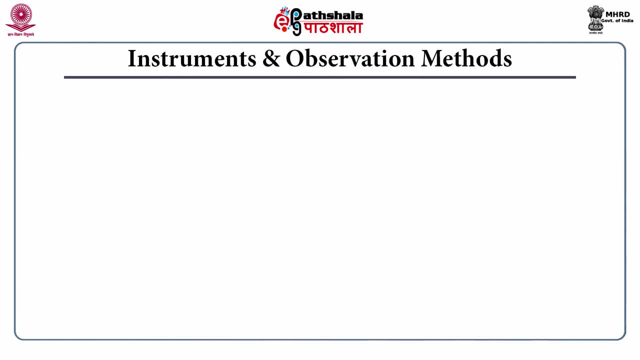 reading of the anemometer, or else it can be taken before commencing of the instrumental observations. Now the various instruments and the observation methods. Let us discuss with wind vane start with wind vane. Wind vane records wind direction. Wind direction is the direction from which. 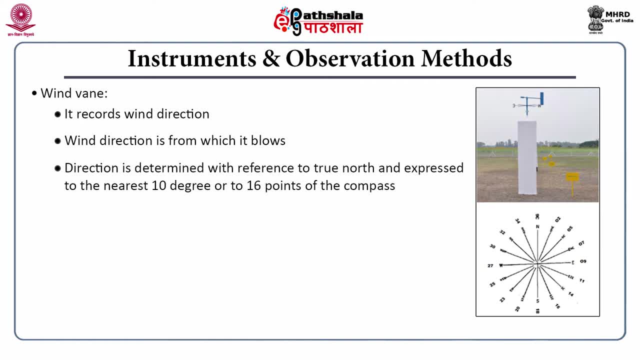 wind blows. Direction is determined with reference to true north and expressed to the nearer 10 degrees or 16 points of the compass. This instrument is a balanced lever which turns freely about a vertical axis Like an arrow. the one end is like an arrow and the other 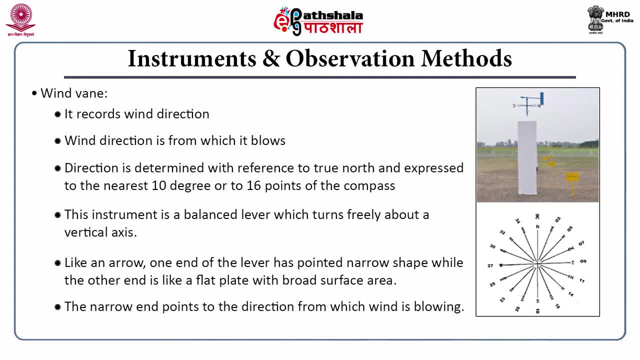 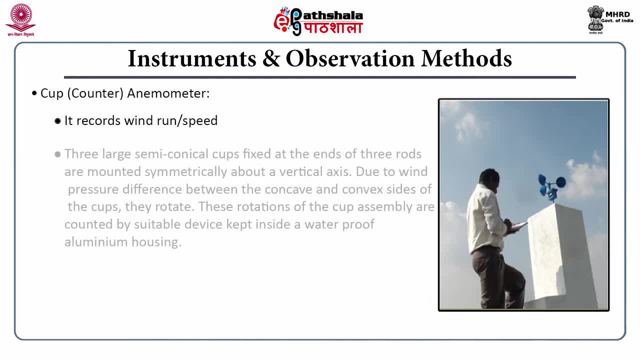 end is like a flat plate, So the narrower end points to the direction from which wind is blowing. Next comes cup anemometer. It records wind run. There are 3 large semi-conical cups fixed at the ends of 3 rods and these are mounted symmetrically about a vertical 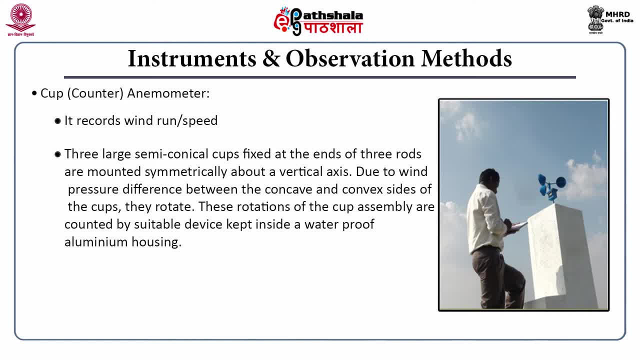 axis, So the wind pressure difference between the concave and convex sides of the cups they rotate. These rotations of the cup assembly are counted by suitable device kept inside a waterproof aluminium housing. The counter is read at the beginning and end of a period. 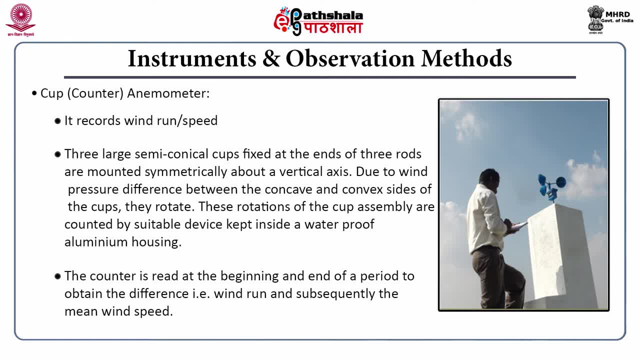 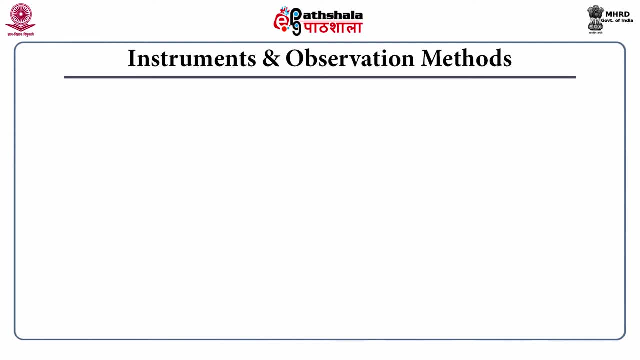 to obtain the difference that is the wind run, And then if we divide the wind run by the time period, then we can get mean wind speed. Next equipment is Dien pressure tube- anemograph. Wind pressure pressure tube- anemograph- Wind pressure pressure tube- anemograph Wind. 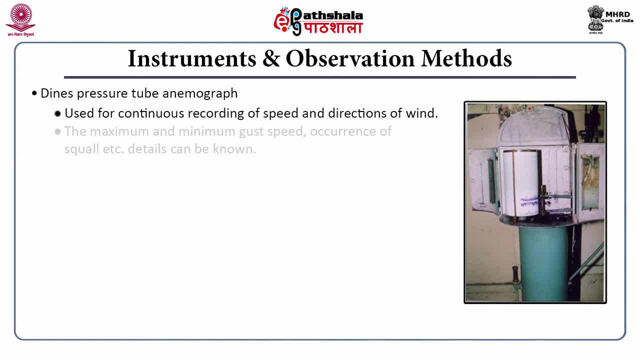 recording of wind speed and directions of wind. The details of wind structure can be known from this kind of equipment, like the occurrence, time of occurrence of maximum and minimum gust speed, then occurrence of squall, etcetera. The direction is measured and recorded by wind vane and a mechanical twin-pane recorder. In case of speed, it is measured by pyrotic. 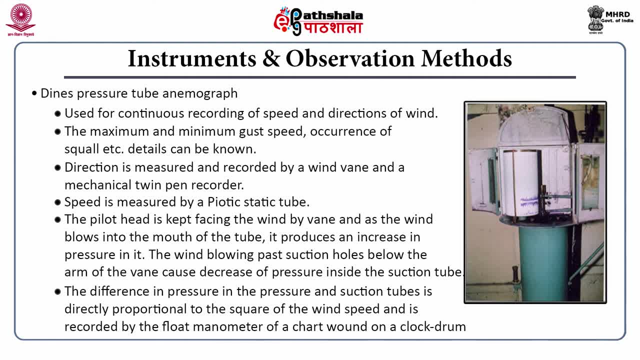 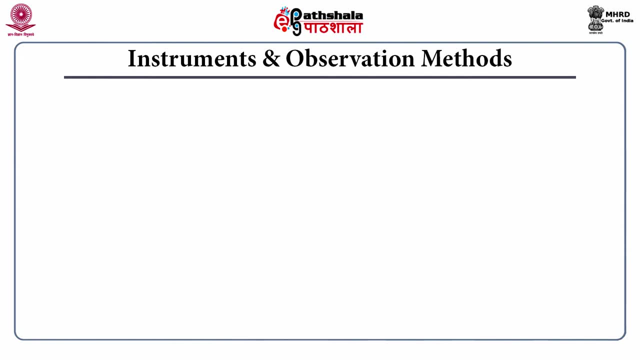 static tube. The difference in pressure in the pressure and suction tubes of this equipment is directly proportional to the square of the wind speed and is recorded by a float manometer, that is, on a chart which is wound on a clogged drum. The next equipment is ordinary rain gauge. It measures the total amount of rain for a. 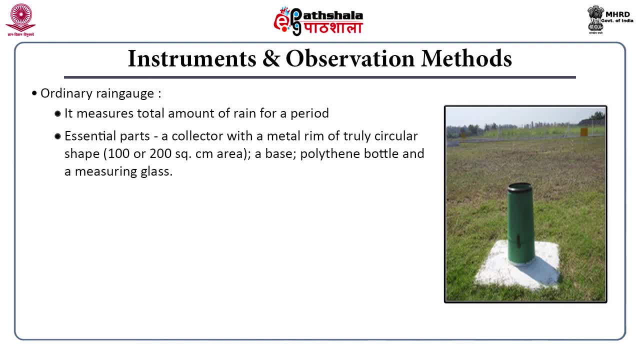 given time period. The essential part of it is a collector with a metal rim of truly circular shape. The size is generally 100 to 200 square centimeter. Then there is a base, a polythene bottle And a measuring glass. The collector and the base are made of FRP, that is, fiber glass reinforced. 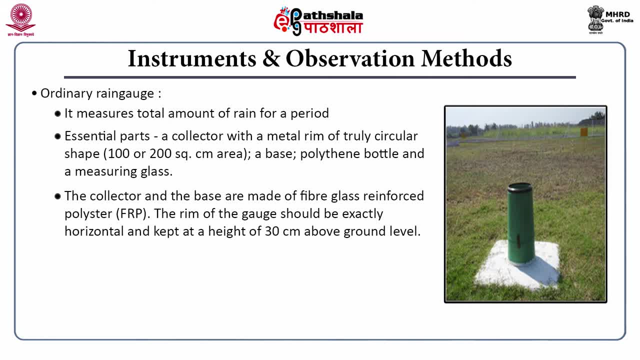 polyester. The rim of the gauge should be exactly horizontal and kept at a height of 30 centimeter above the ground. To measure the rainfall. remove the funnel or collector of the rain gauge, Then take the liquid in a polythene bottle and pour its content in. 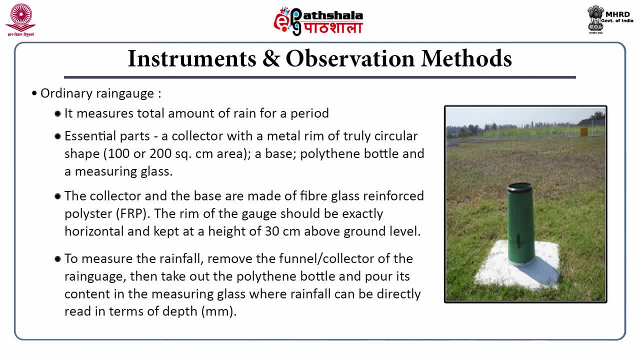 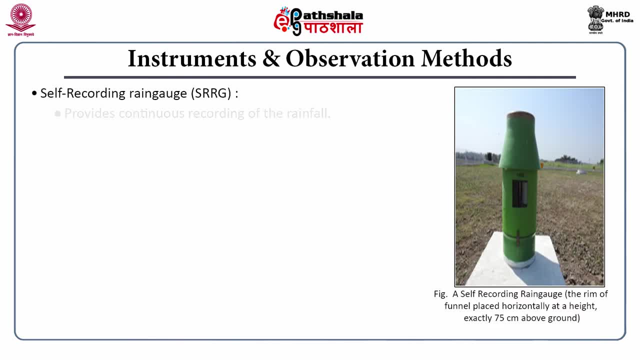 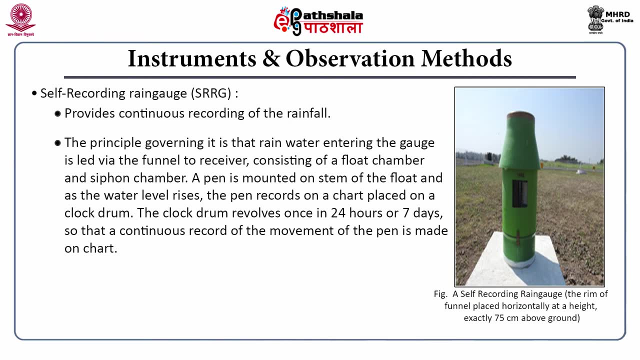 the measuring glass. In the measuring glass it is already graduated and the depth of the rainfall can be directly read. Then comes self recording rain gauge. It provides continuous recording of the rainfall. The principle governing it is that rain water entering the gauge via 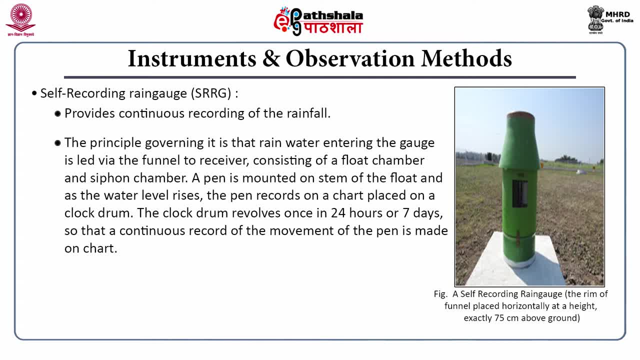 a funnel to a receiver. The receiver consist of a float chamber and a siphon chamber. The pen is mounted on stem of the float And, as the water level rises, the pen records on the chart, which is placed on a clogged drum. The clogged drum revolves once in 24 hours. 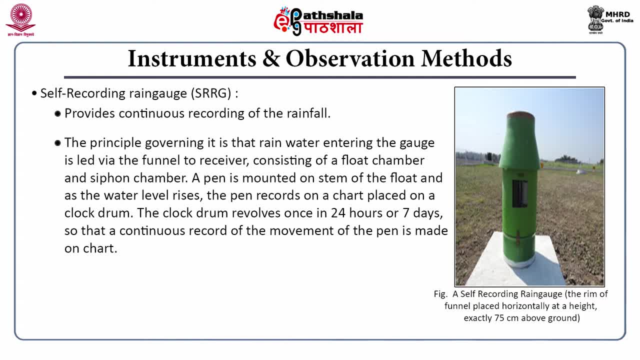 or 7 days, so that a continuous record of the movement of the pen is made on the chart. Once the automatic siphoning occurs, once the pen reaches the top of the chart, and as the rain continues, the pen rises again from the zero line. 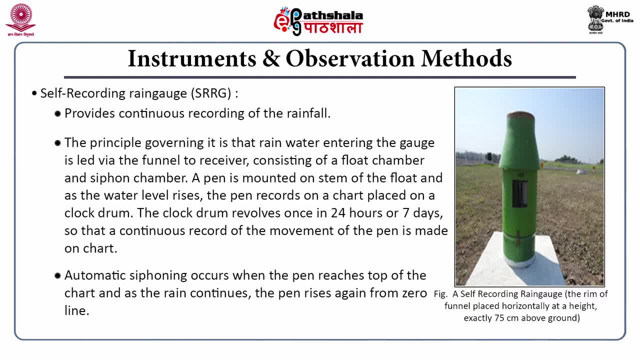 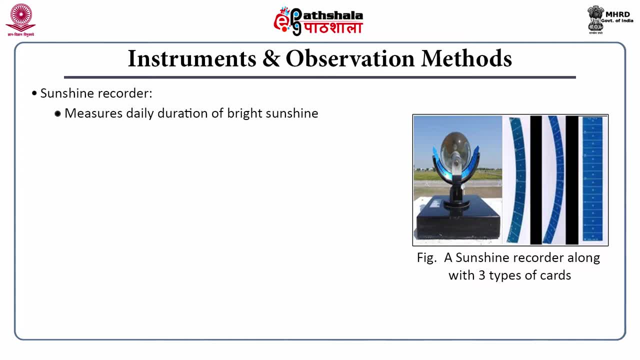 If there is no rain, then the pen traces the horizontal line. Next equipment is sunshine recorder. It measures the daily duration of bright sunshine. It consists of a glass sphere which is about 10 cm in diameter. This glass sphere is mounted concentrically in a section of a hemispherical bowl which 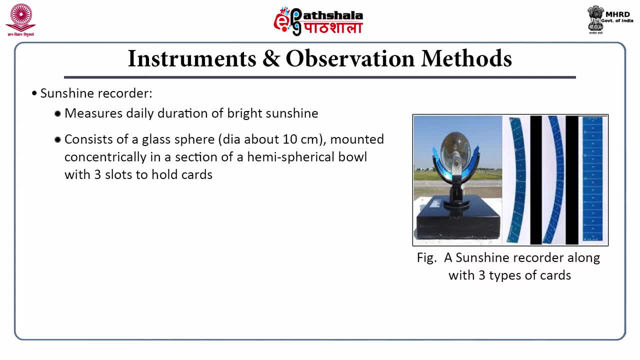 has three slots to hold three different type of card. During summer time, long curved card is used and this is put at the bottom slot. The time during which it is used is 13th April to 31st August. The next type of card is short curved card. 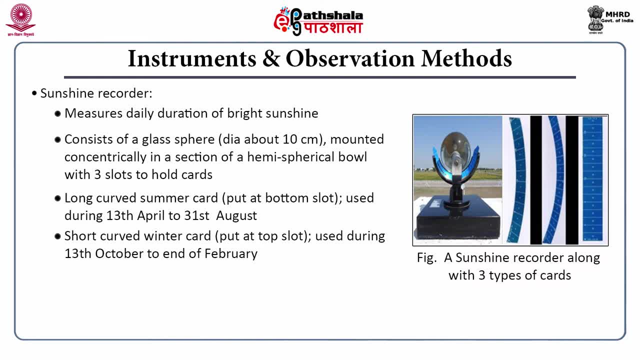 It is used during winter time and it is put at the bottom slot. The time during which it is used is 13th October to end of February. The third type is straight or equinoxial card. It is put at the middle slot and used during 1st March to 12th April and then 1st September. 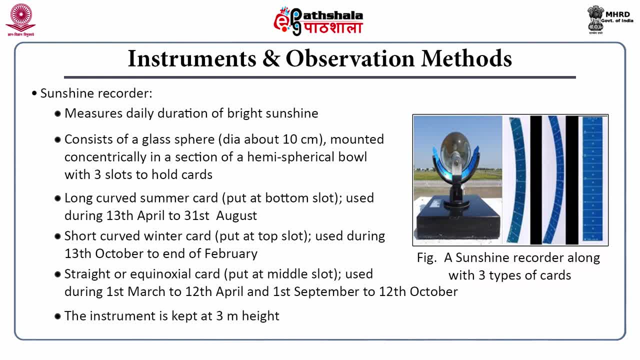 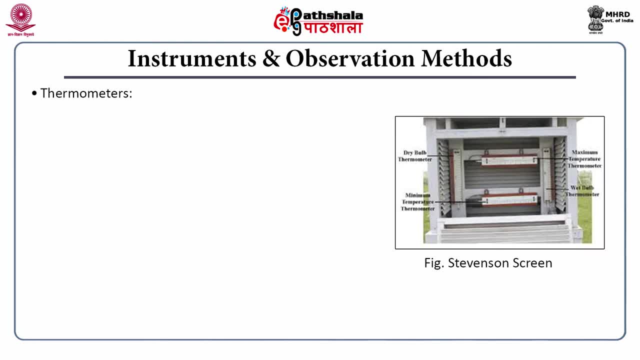 to 12th October. The instrument is kept at open, exposed place at 3 meter height. Then comes thermometer. There are four type of thermometer: Maximum, minimum thermometer and drivable orbital thermometer. The instrument is kept at open, exposed place at 3 meter height. 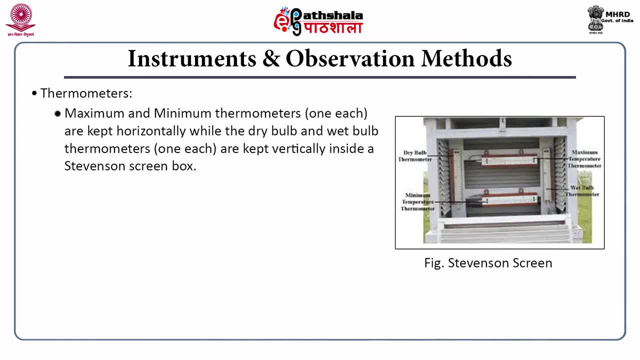 Then comes thermometer. These are kept inside a Stevenson screen. The Stevenson screen is a rectangular box with a sides and door double word and the roof is double layered. The base of the box is at 1.25 meter height and door opens to the north. in the northern 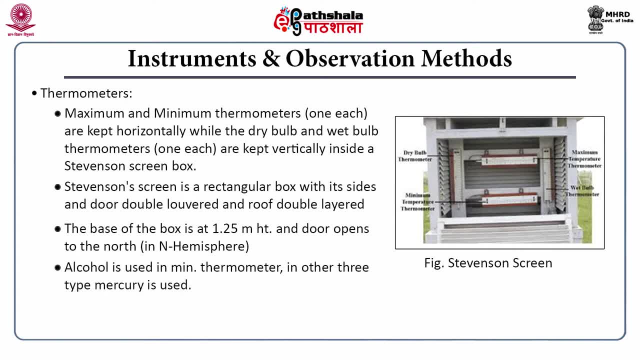 hemisphere. Such arrangement is to avoid the exposure of direct sun, because the thermometers are meant for not the temperature of direct rays of sun. In all the types of thermometers, mercury is used as a sensing element, But in case of minimum thermometer, alcohol is used. 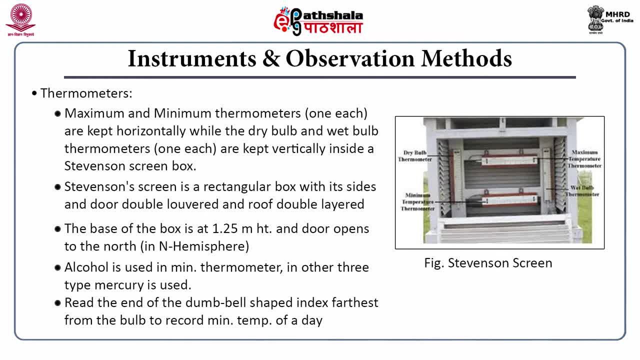 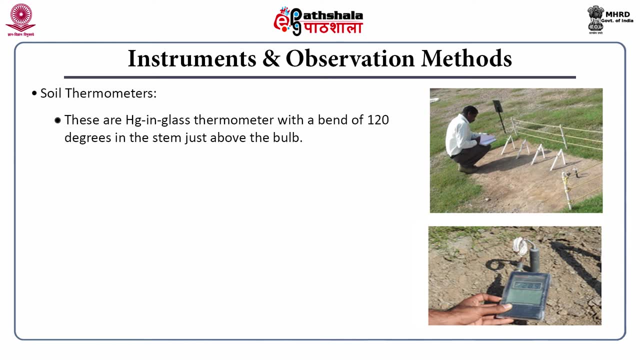 There is a dumbbell shaped index inside your minimum thermometer and we should read the end, which is furthest from the bulb, to know the minimum temperature for a given time period. Now comes soil thermometers. These are also mercury in glass thermometer which has a bend of 120 degree in the stem. 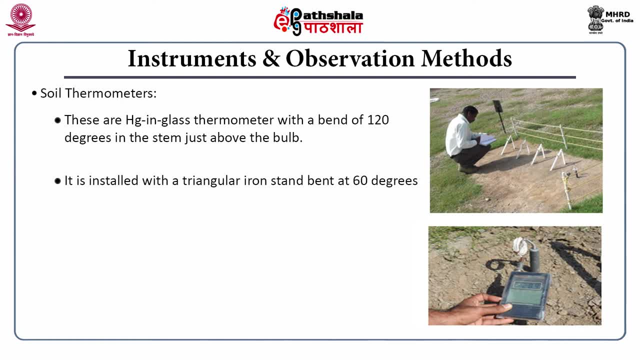 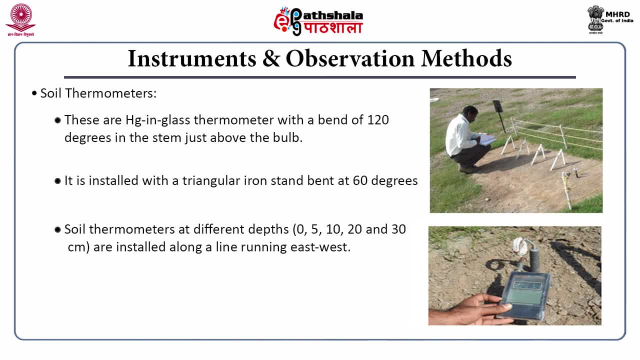 20 centimeter and 30 centimeter. These are installed along the line running east to west and the measurement is meant up to 30 centimeter because variations can be seen beyond that depth. The variations are generally less and generally not measured. Soil temperature probes with digital meters are also nowadays used to record soil temperature. 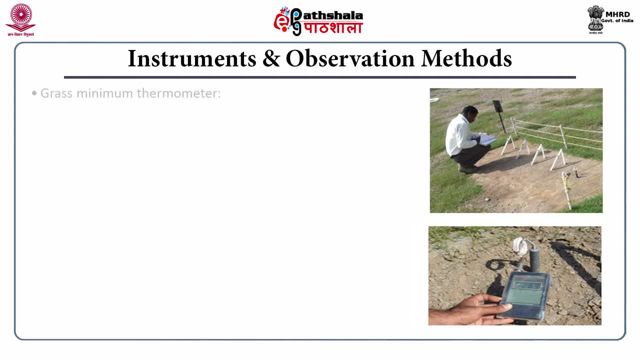 used to record soil temperature. Next is grass minimum thermometer. It is also known as terrestrial radiation thermometer. It is used to obtain information about the occurrence of ground frost at night. The instrument is exposed on a plot covered with a short grass 2.5 to 5 centimeter height. 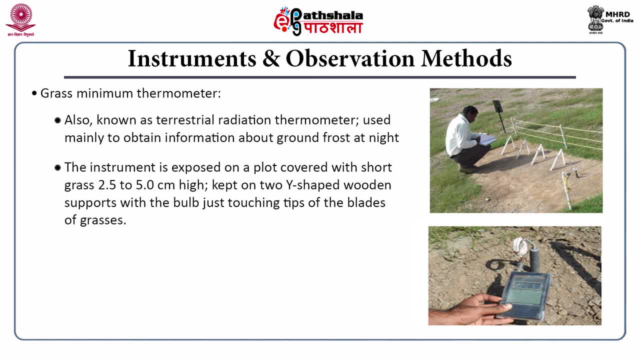 It is kept on two y-shaped wooden supports with the bulb just touching the tips of the blade of the grass. It should be read at the hour of routine morning observation. After the reading is over, the thermometer is kept inside the screen with bulb downwards. 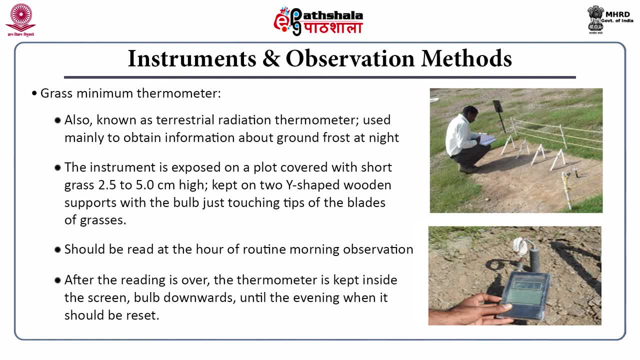 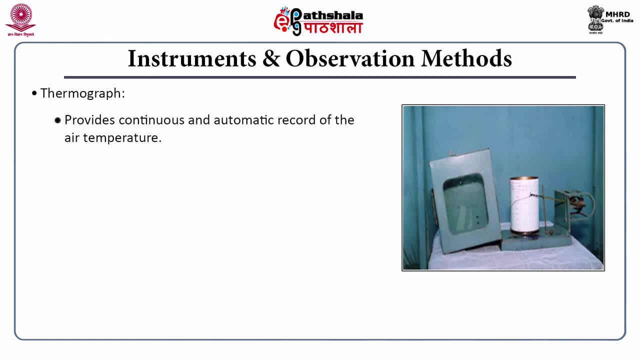 until the evening. During evening time it is set again and put over the grass. Thermograph provides continuous and automatic record of air temperature. It is placed inside the double estimation screen. Thermograph has a temperature sensing sensitive element. generally a bimetallic strip is used. 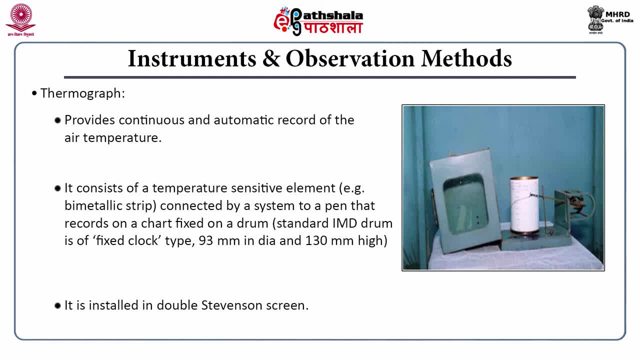 as a sensor And it is connected by a system To a pen. that pen records on a chart which is fixed on a drum. Standard IMD drum is a fixed clock type. They have diameter of 93 millimeter and 130 millimeter in height. 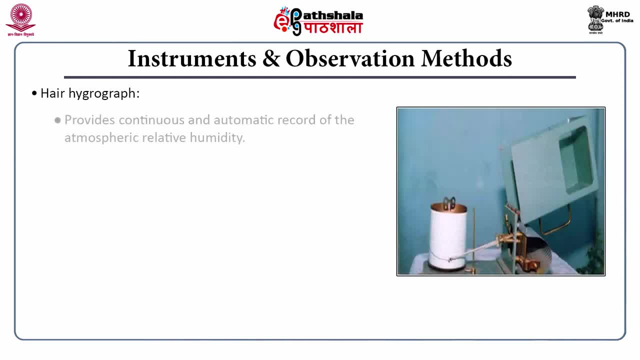 The next equipment is air hygrograph. In case of air hygrograph, air is used as a sensing element because human ear is sensitive to relative humidity of the air. Its length changes Proportional to the logarithm of the changes in the relative humidity. 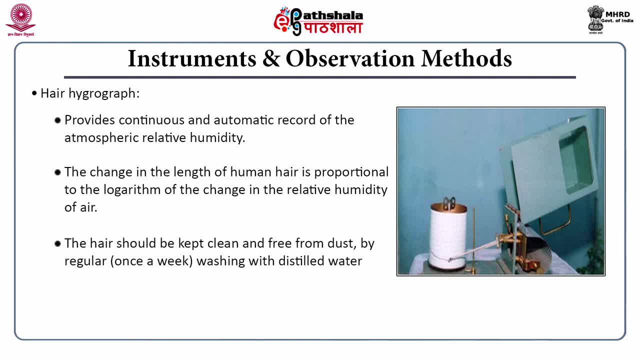 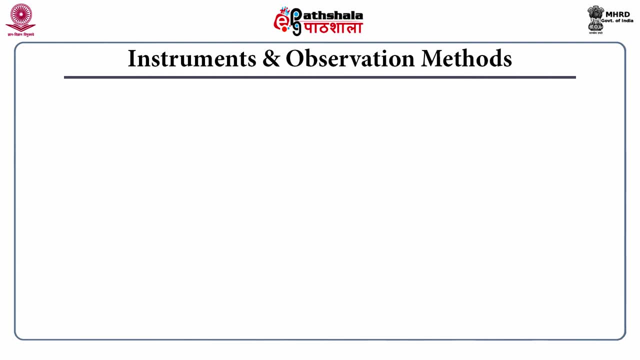 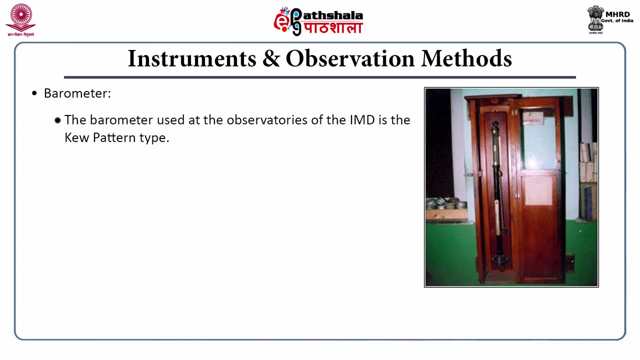 The air should be kept clean and free from dust. It should be regularly washed with distilled water. This equipment is also placed inside the double estimation screen. Our next equipment is barometer. Barometer is used to measure air pressure. There are different types, but in most of the IMD observatories Q pattern type barometer. 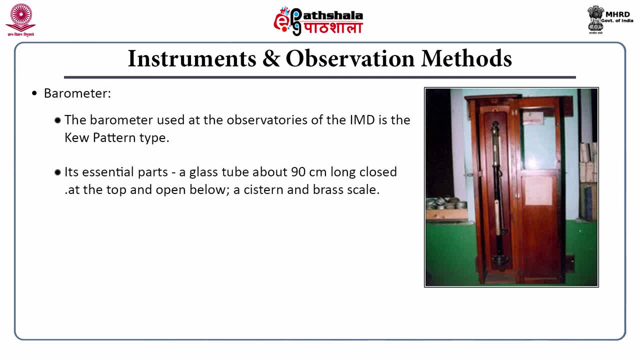 is used. Its essential part is a glass tube. Above the barometer is a glass tube. It is used to measure air pressure. It is about 90 centimeter long. The tube is closed at top end and its open is below. Then there is a cistern and a brass scale. 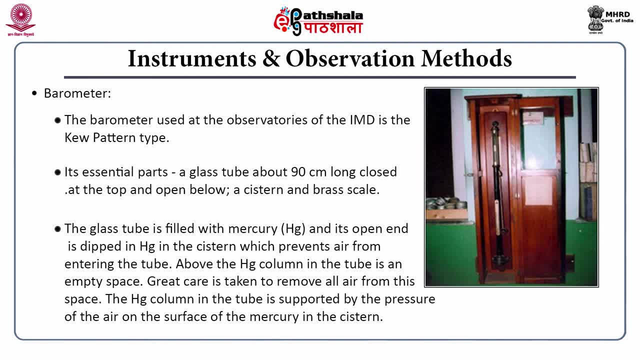 The glass tube is filled with mercury and its open end is dipped in the mercury in the cistern, which prevents air from entering the tube. Above the mercury column in the tube there is an empty space and care should be taken to remove all the air from this space. 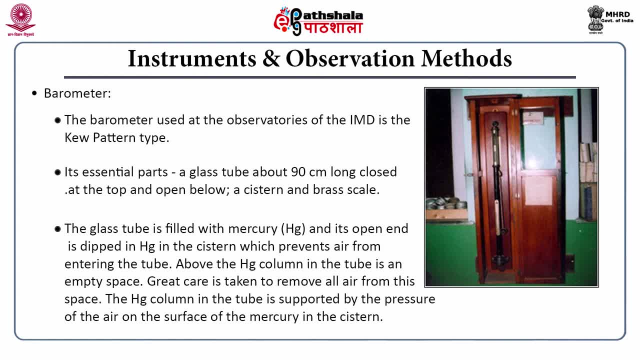 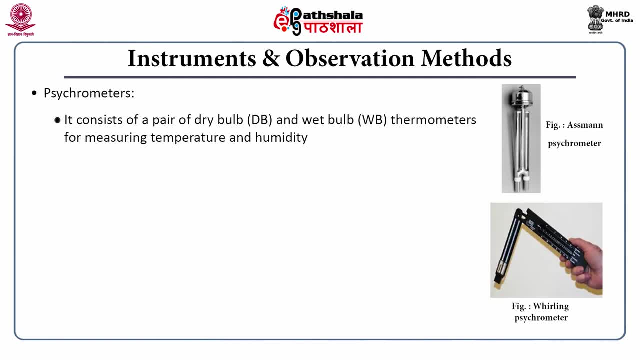 The mercury column in the tube is supported by the pressure of the air on the surface of the mercury in the cistern. Next equipment is psychrometers- Psychrometers generally. it is a pair of dry valve and wet valve thermometers. 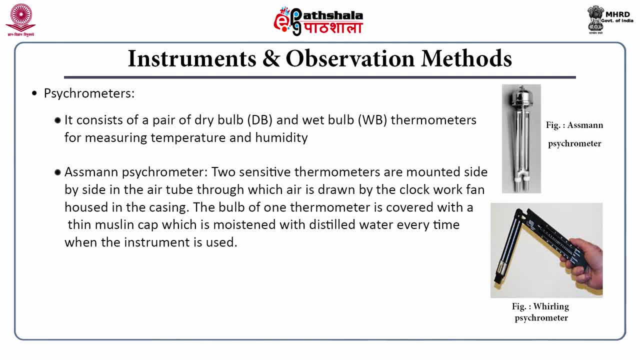 It is used for measuring temperature and humidity. There are two main types. One is Osmond psychrometer, another is Whirling type psychrometer. In case of Osmond psychrometer, this dry valve and wet valve is there and air is sucked. 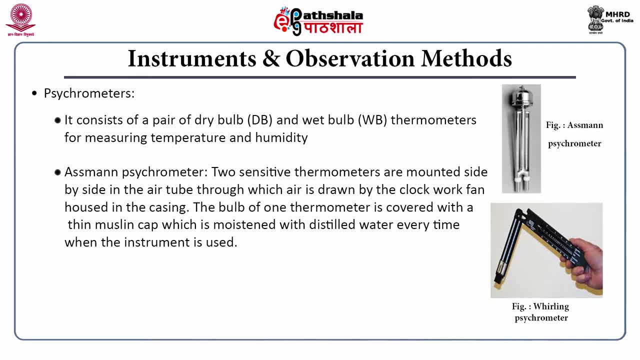 clogged with fan. The tube valve of one thermometer is covered with a thin muslin cap. Each time the psychrometer is used, it should be wetted with distilled water. In case of Whirling psychrometer, aspiration is provided by whirling or rotating the thermometers. 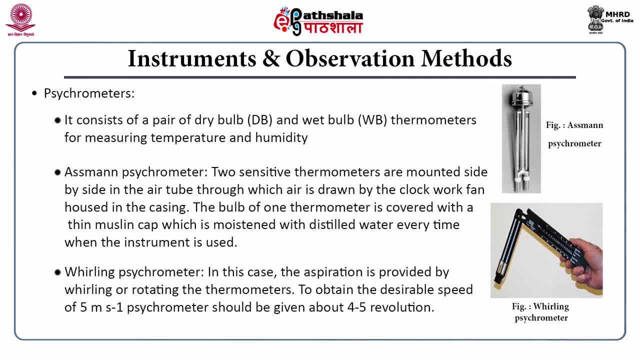 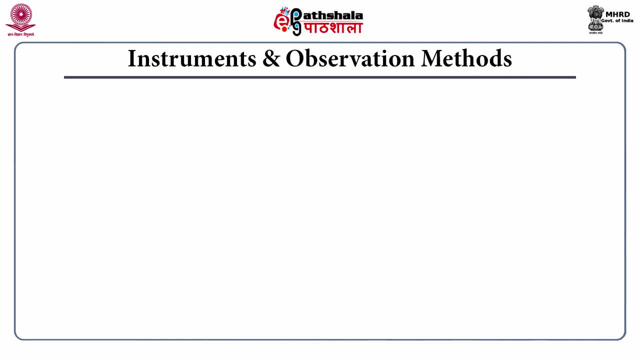 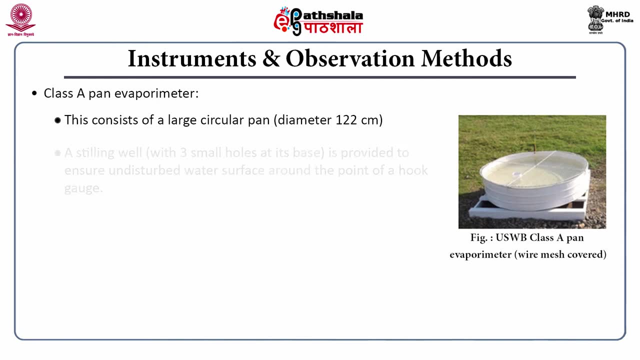 Desired speed is 5 meter per second, which can be obtained by giving 4 to 5 revolutions to this psychrometer. Next equipment is class A pan evaporometer. This consists of a large circular pan with a diameter of 120 centimeter. A steeling well is provided. 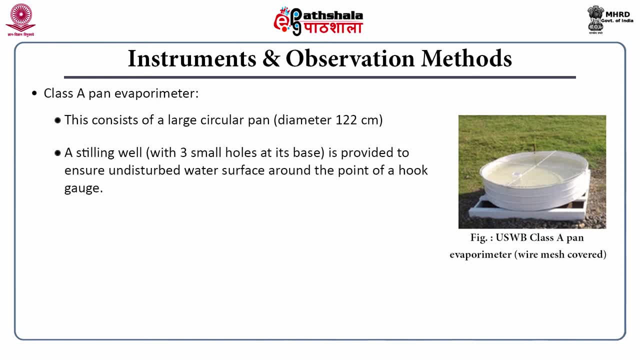 The pan is placed on top of the evaporometer. The pan is placed on top of the evaporometer. The pan is placed on top of the evaporometer. It has three small holes at its base. The steeling well is provided to ensure that there is no ripple on its surface. 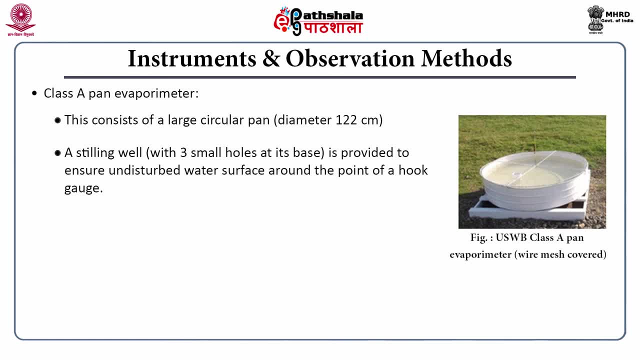 So that the level of water can be accurately read. The amount of water lost by evaporation from the pan during any interval of time is measured by adding known quantities of water to the pan from a graduated cylinder whose diameter is 1 tenth that of the diameter of the open pan. 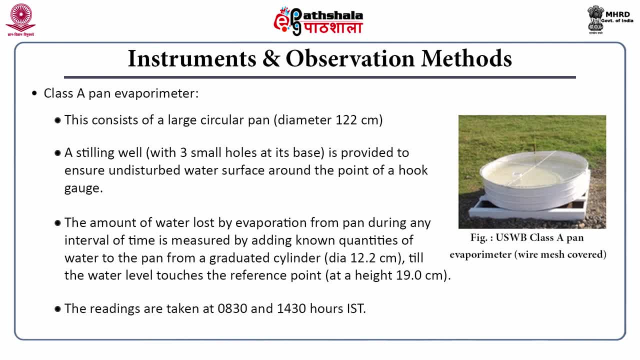 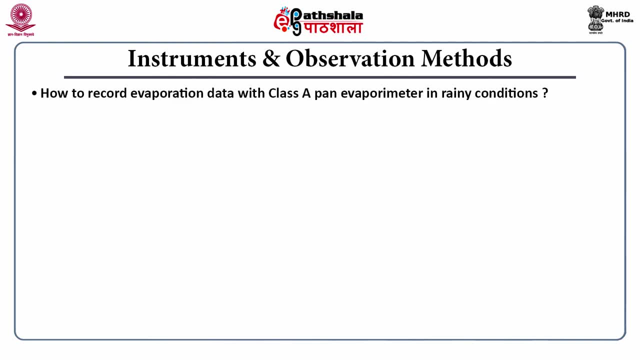 The readings are taken generally at 830 hours IST and in some observatory a second observation at 1430 hours is also taken. Now, how to record evaporation data with a class A plan evapometer when there is a rainy condition. Now there could be light rainy days. there could be heavy rainy days. 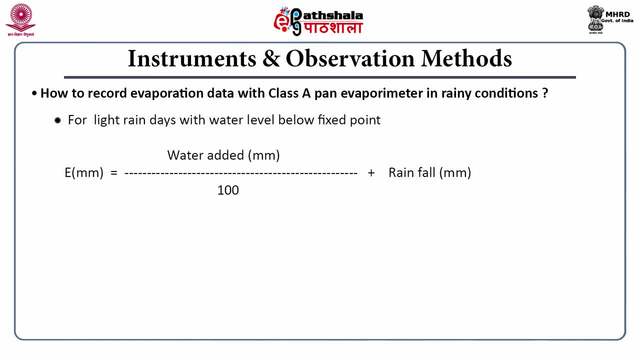 During light rainy days, when water level is still below the tip of the hook gauge or the reading point, this formula is used. It is: evaporation is equal to water added in millimeter divided by 100, plus rain in millimeter For heavy rainy days, when we need to remove water to get the water level up to the tip. 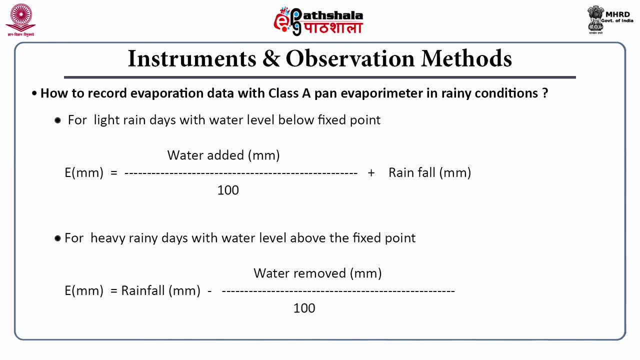 of the hook. we need to use this formula: Evaporation is equal to rainfall minus water removed divided by 100.. Our next document is Duke-Dubony-Dugas. It uses wooden blocks of 32 by 5 by 2.4.. 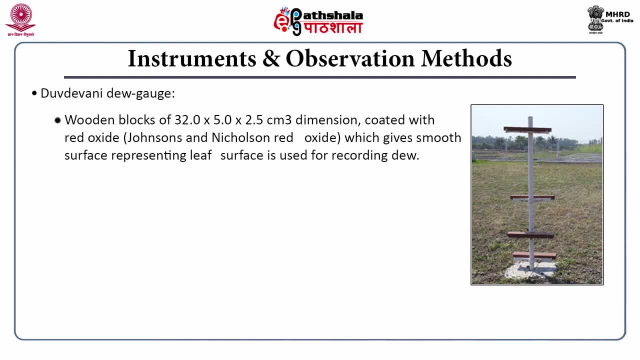 It is a 5 centimeter cube dimension which is coated with red oxide. The chemical is Johnson's and Nicholson's red oxide. This coating is done to give it a smooth surface so that it can represent the leaf surface. The dew gauges are kept at different heights, namely 5 centimeter, 25 centimeter, 50 centimeter. 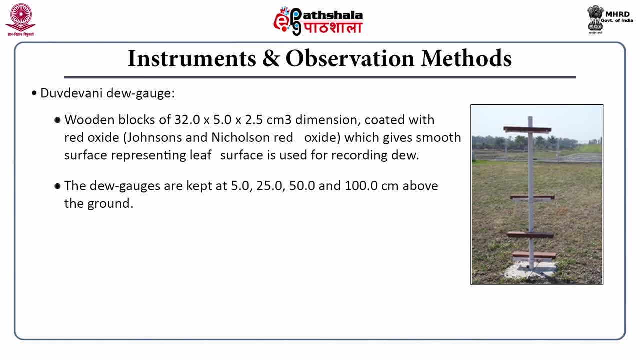 and 100 centimeter above the ground. The instrument is set after sunset and the observation is taken just before the sunrise Because if you delay then sunrise will cause the evaporation of the dew and we will not get the actual measurement. The amount of dew over the dew gauges are compared to the standard dew photographs. 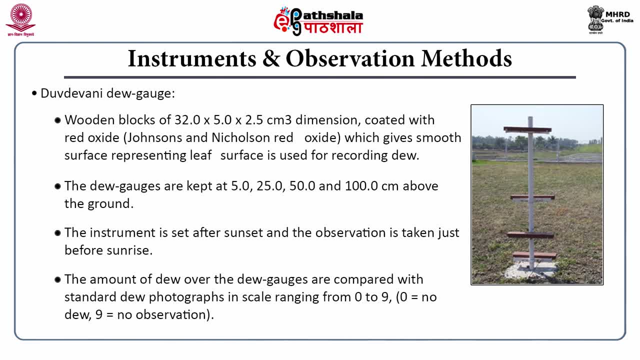 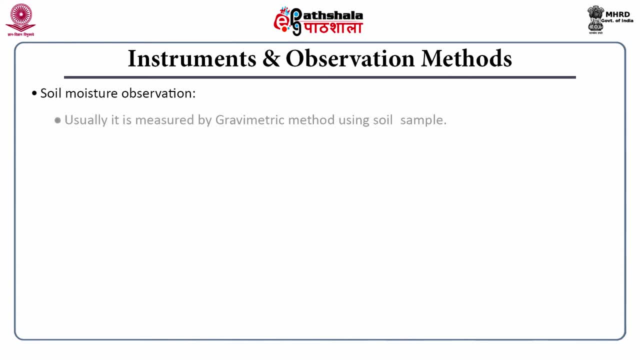 which, in scale ranging from 0 to 9.. 0 means no dew and 9 means no observation. Now soil moisture observation is taken in most agro-matter observatories. It is usually measured by gravimetric method. Soil samples are collected in aluminum boxes. 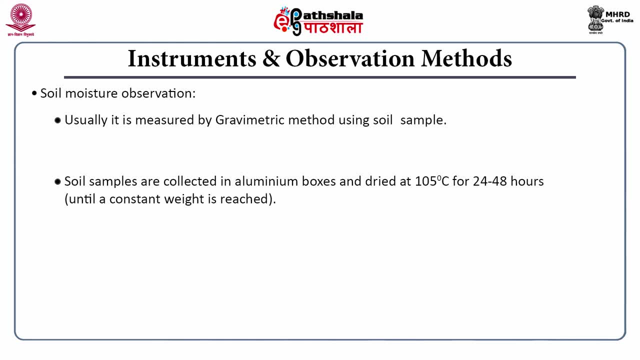 And those are dried at 105 degree centigrade till a constant weight is reached, Generally based on soil and moisture content. 24 out of 48 hours is required to attain this constant weight And moisture content is calculated using the following formula: 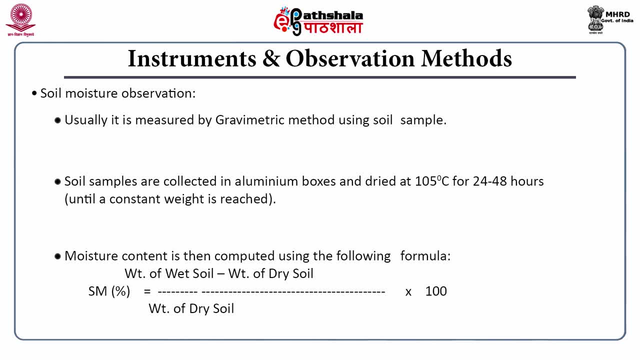 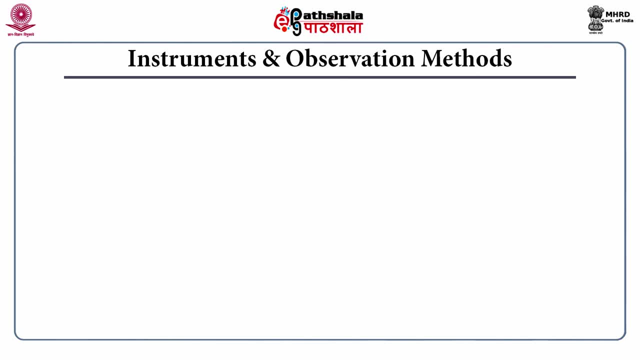 Soil moisture content percentage. gravimetric moisture content is weight of wet soil minus weight of dry soil, divided by weight of dry soil into 100.. Now the non-instrumental observations. The non-instrumental observations. The non-instrumental observations. 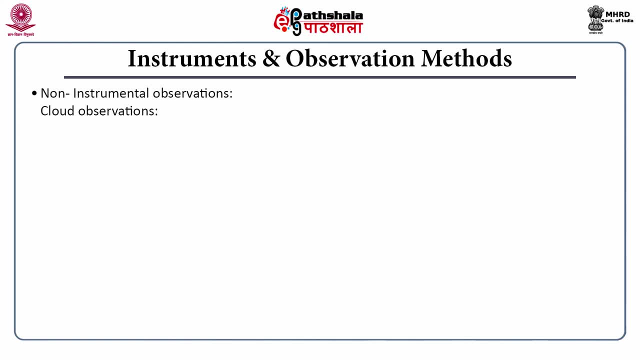 That means observations which do not require instruments. Without the aid of the instruments also, these parameters can be measured. One of them is cloud. The cloud amount is reported in terms of octa. If the sky is completely cloudless, then it is 0 octa. 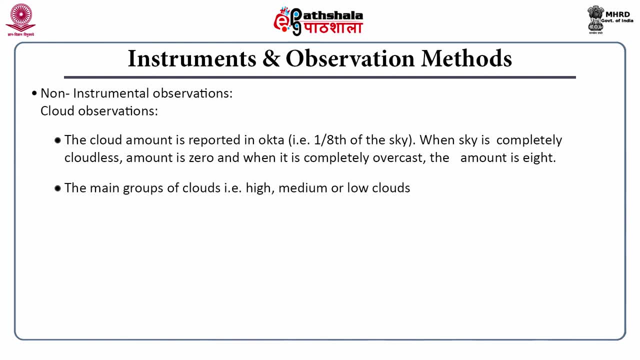 If it is completely overcast, then it is 8 octa. Then main groups of clouds can also be identified, like high cloud, medium cloud or low clouds. Then cloud height: That is the height of the base of the cloud from the ground. 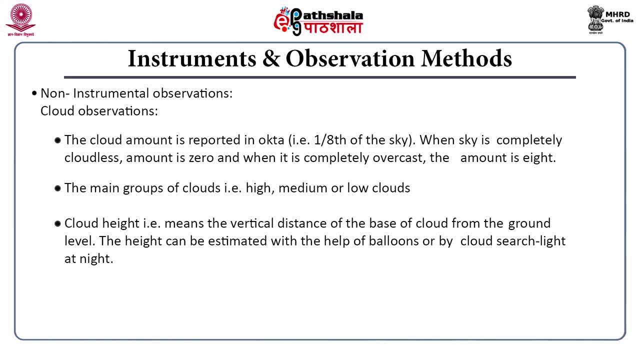 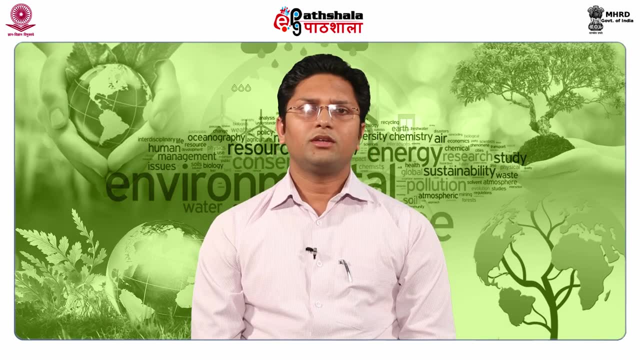 It can be measured, estimated with the help of balloons or, during night time, by search light. also it can be estimated. The direction of movement of cloud is usually can be visually estimated nearest to the eight point of the compass. To summarize, there are six classes of surface meteorological observatories and the data. 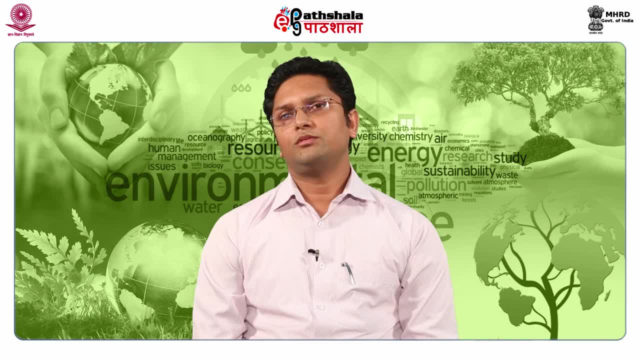 recorded in all the observatories at a standard prescriptive level. So this is the first class of surface meteorological observatories and the data recorded in all the observatories at a standard prescriptive level. First class is skyward hours- Data recorded in the following order: 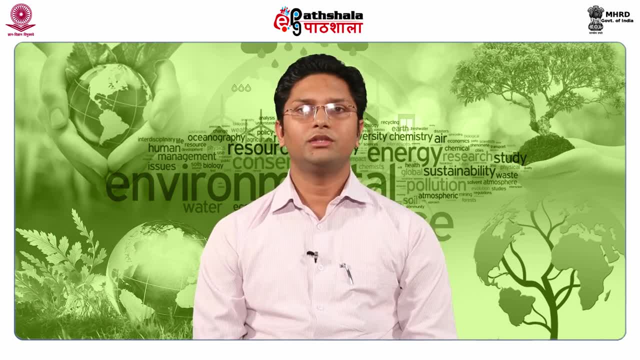 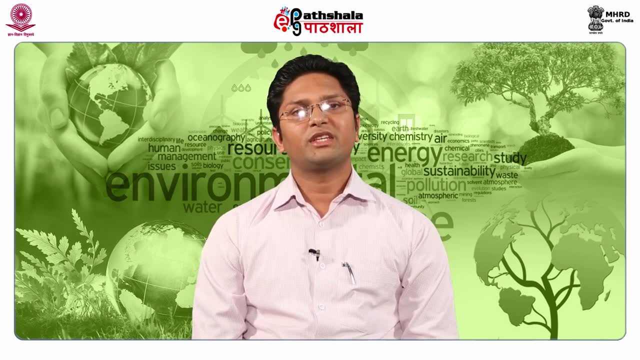 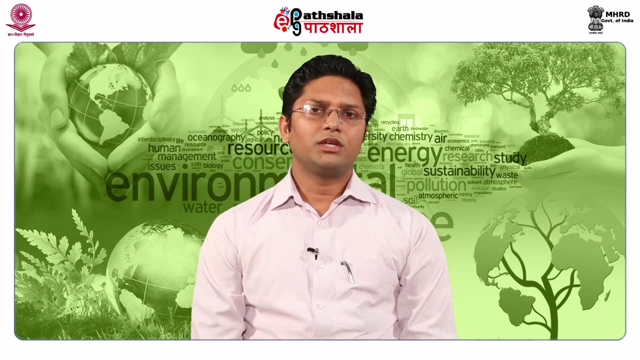 First wind instruments, following by rain gauge, then thermometers, then barometer. The wind direction and the speed are recorded using wind vane and copper neighbors respectively, The maximum-minimum dry-valve and weed valve. thermometers, along with thermographs are used to record temperature. 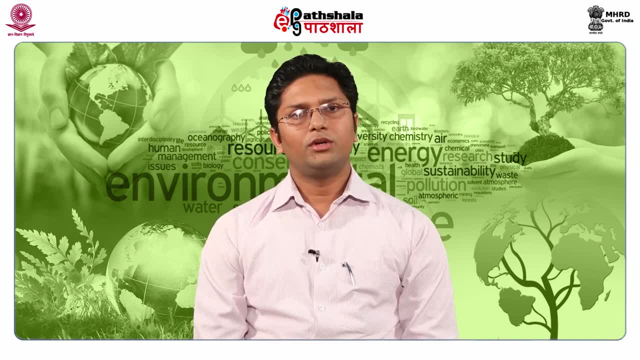 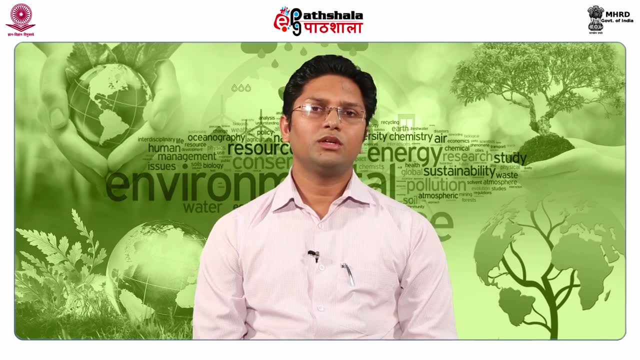 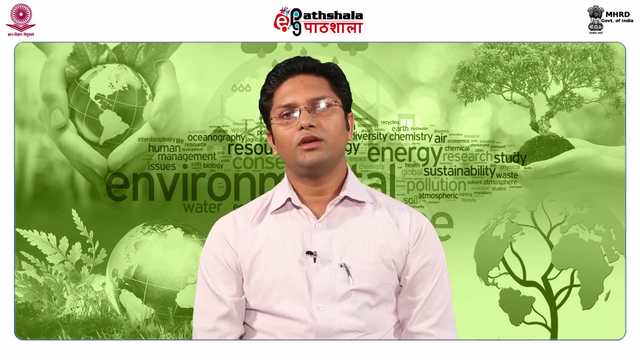 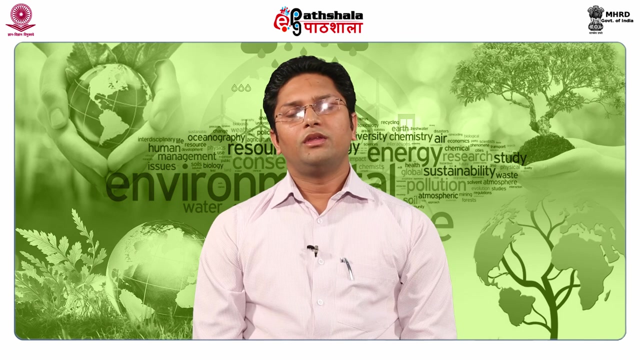 Sunshine recorder is used to record bright sunshine over the duration. Soil temperatures are measured at different depths. Grasp minimum thermometer is used for information about ground frost. psychrometers and hygrographs, along with your dry bulb and wet bulb thermometers, are used for computations of relative humidity.